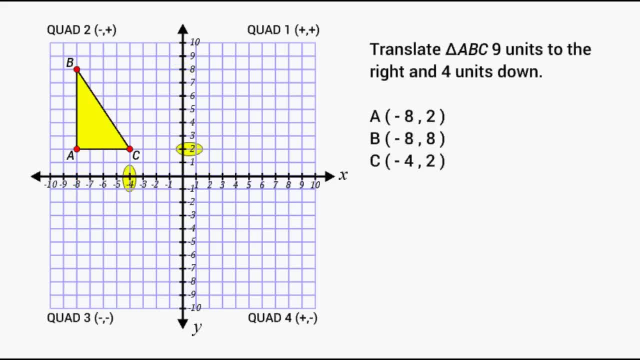 And point C is located at negative 4, positive 2.. Now we are being asked to translate our triangle 9 units to the right. Any movement to the right on the coordinate plane is a positive movement in the x direction. That just means. 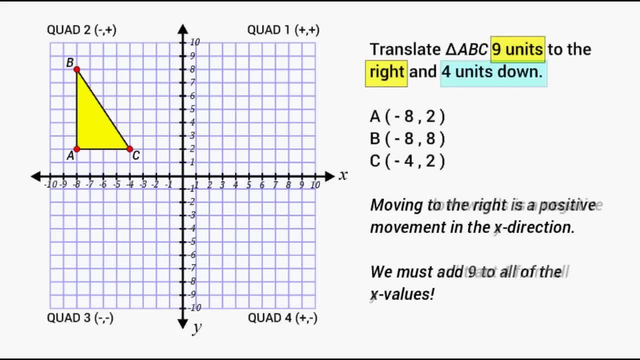 we have to add 9 to all of our x values And we have to translate this triangle 4 units down as well. Any movement downward is going to result in a negative movement in the y direction. Therefore, we're just going to subtract 4 from each y value. So first let's add 9. 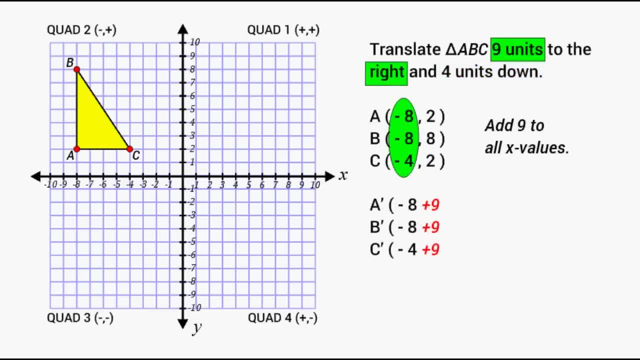 to each x value. Negative 8 plus 9 is positive 1. Negative 8 plus 9 is also positive 1. And negative 4 plus 9 will result in positive 5.. Now let's subtract 4 from all of our 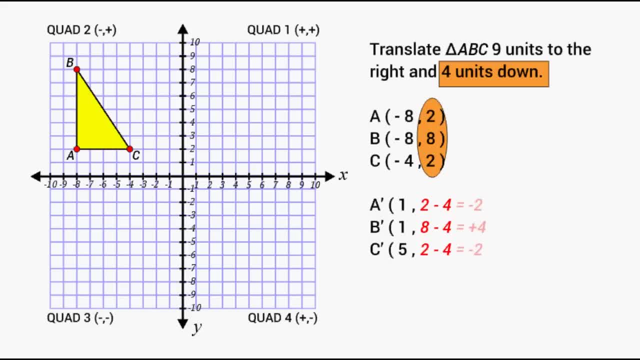 y values: 2- take away 4 is negative. 2.. 8- take away 4 is positive. 4. And 2- take away 4 is negative, 2.. So, after adding 9 to all of our x values and subtracting 4 from all of the y values, 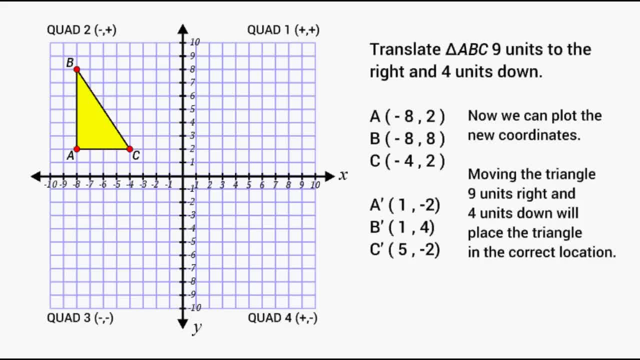 we will come up with the coordinates to where our object is going to be translated to, So we can simply plot those points and then create our new object on the coordinate plane. So what we're going to do is we're going to just take our object and slide it over. 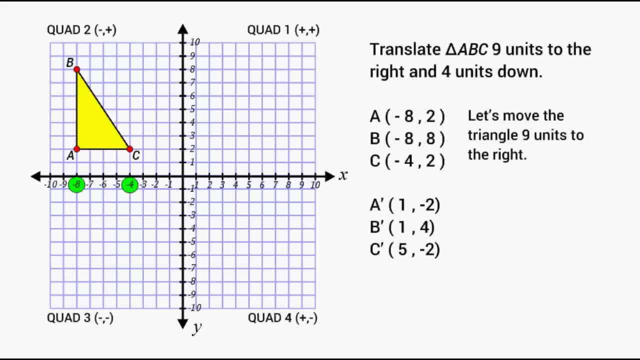 9 units to the right, And then we're going to slide it 4 units down, just to show it will end up in the coordinates that we came up with. Okay, so let's start by moving the triangle to the right And then we're going to slide it 4 units down, just to show. it will end up in the coordinates that we came up with. 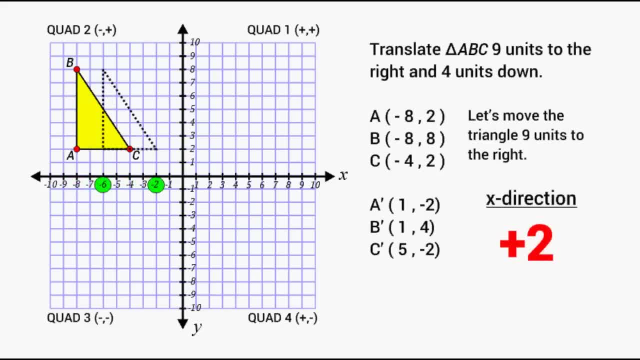 1,, 2,, 3,, 4,, 5,, 6,, 7,, 8,, 9 to the right. All right, now let's slide our triangle: 4 units down: 1,, 2,, 3, and 4 units downward. 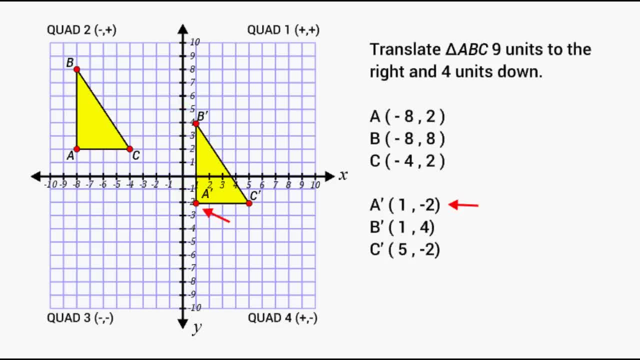 All right, now let's check to make sure that our points are in the correct location. Point A did end up at positive 1, negative 2.. So we're going to slide our triangle 4 units down- 1,, 2,, 3,, 4, 5,, 6,, 7,, 8, 9- to the right. All right, now let's check to make sure that. 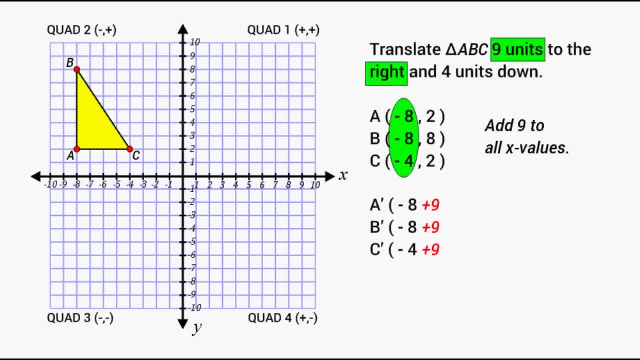 to each x value. Negative 8 plus 9 is positive 1. Negative 8 plus 9 is also positive 1. And negative 4 plus 9 will result in positive 5.. Now let's subtract 4 from all of our 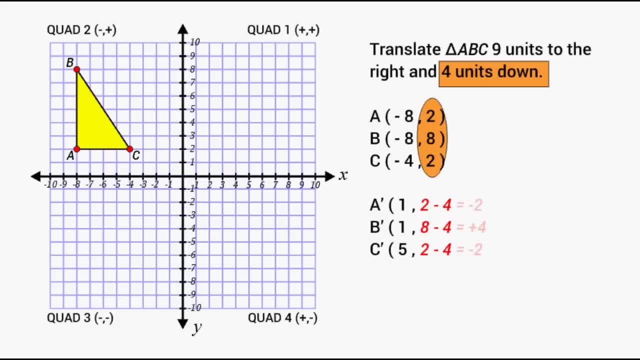 y values: 2- take away 4 is negative. 2.. 8- take away 4- is positive. 4. And 2- take away 4 is negative, 2.. So, after adding 9 to all of our x values and subtracting 4 from all of the y values, we 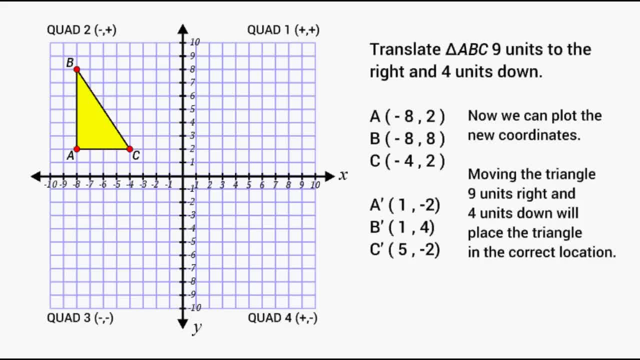 will come up with the coordinates to where our object is going to be translated to, So we can simply plot those points and then create our new object on the coordinate plane. So what we're going to do is we're going to just take our object and slide it over. 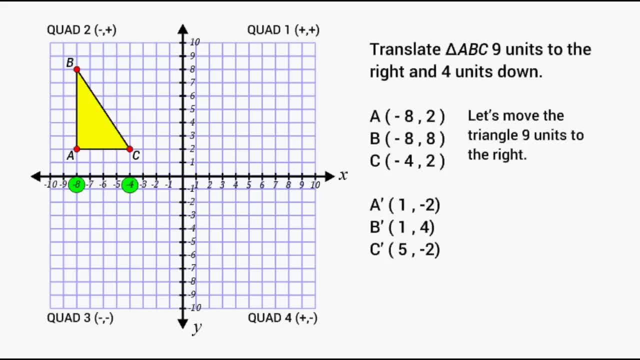 9 units to the right And then we're going to slide it 4 units down just to show it will end up in the coordinates that we came up with. Okay, so let's start by moving the triangle to the right. 1, 2,, 3, 4,, 5,, 6,, 7,, 8, 9 to the right. 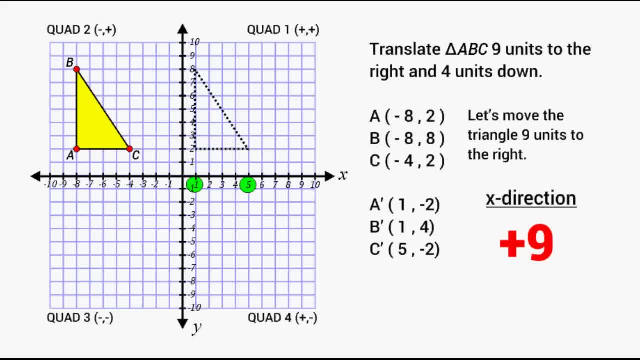 All right, Now let's slide our triangle 4 units down: 1,, 2,, 3, and 4 units downward. All right, Now let's check to make sure that our points are in the correct location. Point A did end up at positive 1, negative 2.. So we're going to slide our triangle 4 units. down 1,, 2,, 3,, 4,, 5,, 6,, 7,, 8,, 9 to the right. All right, So we're going to slide our triangle 4 units down: 1,, 2,, 3,, 4,, 5,, 6,, 7,, 8,, 9 to the 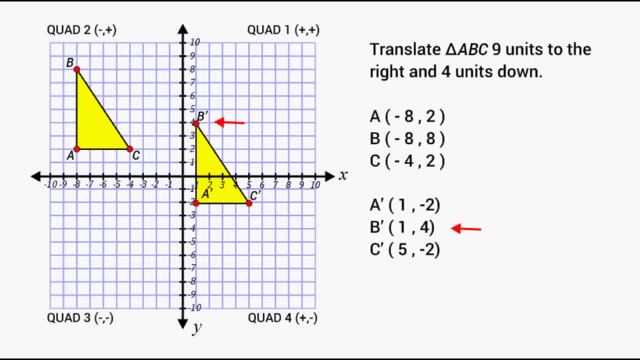 right And point B did end up at positive 1, positive 4.. And point C did end up on positive 5, negative 2.. So we were able to successfully translate this triangle 9 units to the right and 4 units down. 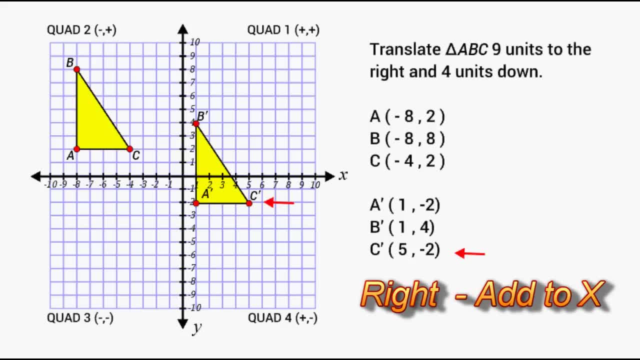 So any movement to the right on the coordinate plane just means you're going to add something to the x value. Now, if you were to move something to the left, then you'd subtract that amount from your x value. Any movement downward is a movement in the y direction and you would subtract from your 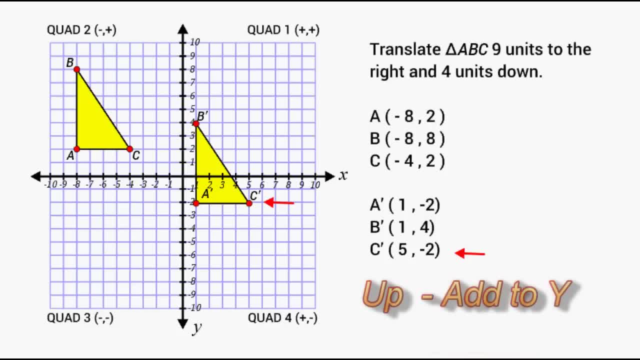 y value And any time you would move something upward, you would end up taking the amount that you moved upward and adding that number to each one of your y values. Hey, I just want to say thanks very much for checking out my math video. Please subscribe.